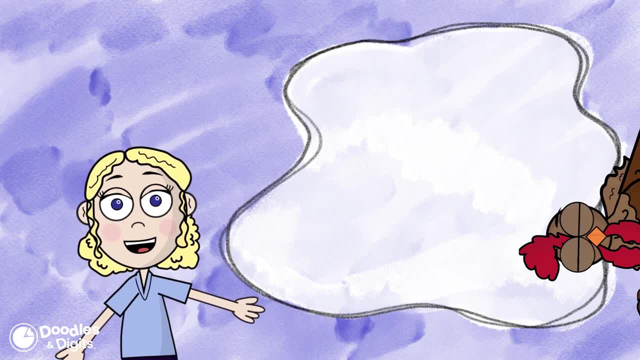 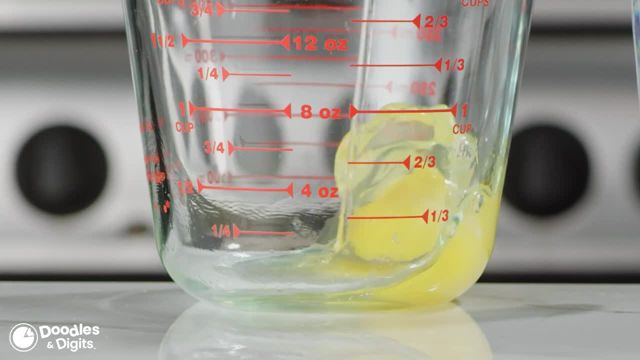 in real life. There are multiple ways you're going to multiply a whole number by a fraction in real life. One of my favorite ways is actually cooking. So, for example, if you need to double or triple a recipe, you're going to have to multiply those fractions of different measurements by whole. 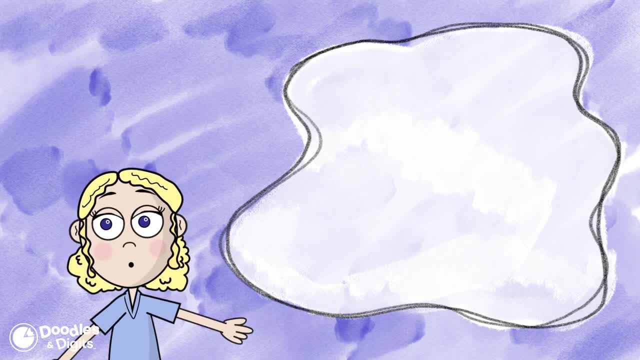 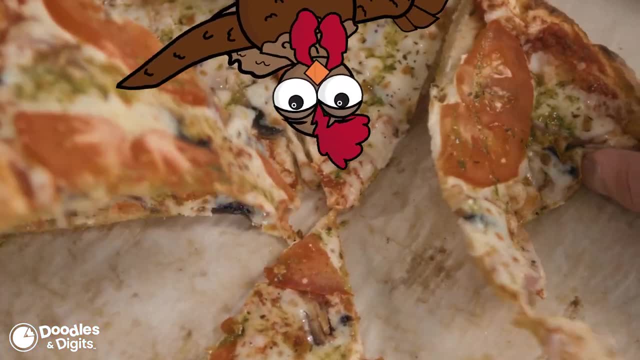 numbers. Another real life example might be when you're sharing. So let's say you cut a piece of pizza into sixteenths and each person has three pieces. When you multiply a fraction by a whole number, you'll be seeing how much each person can eat. So you can see how much each person can eat. 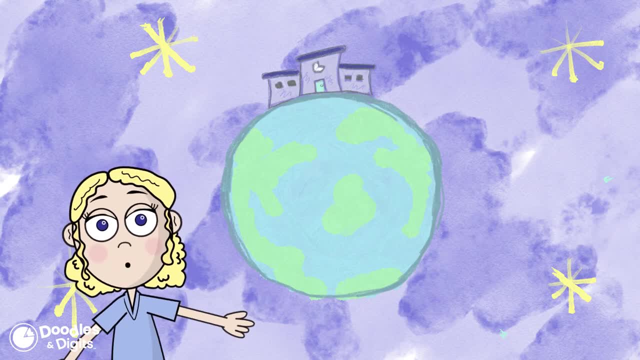 One, except for when I had pizza, which was 23 minutes ago. you can probably see some of that being a że and out of the blue. Then some is being eaten And then another one being eaten. So really that's a really important example. When you multiply a fraction, a whole number, 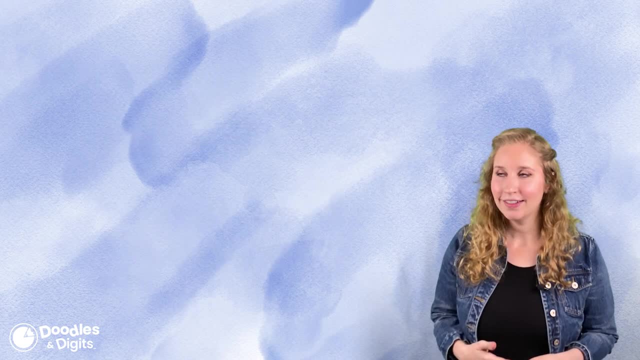 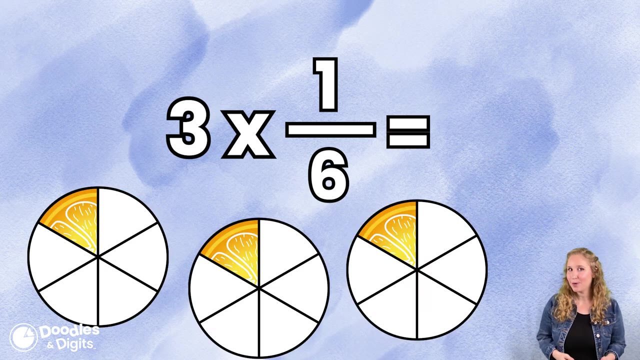 by a fraction is what we're going to do- to how to multiply it between two different types of mixes. So we need to now use this to understand multiplicative model. Let's look at some Engineering exercise. right here We're not going to show you how Milli and working with We, 나�a to select. 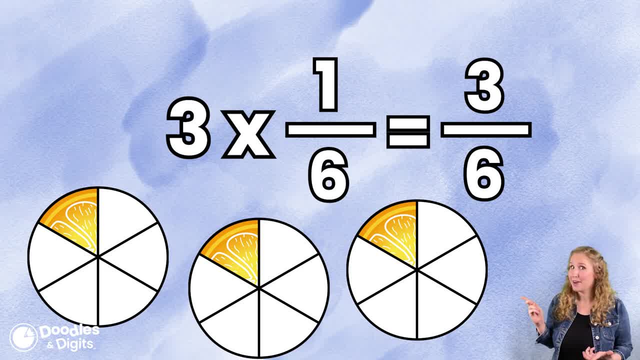 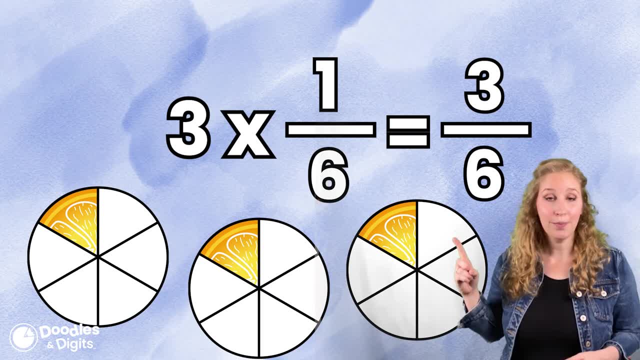 üç in one household and then solve our answer way in real life is either by a fraction or a whole number. you might have noticed, when we multiply a fraction by a whole number, we're gonna actually multiply the numerator and keep the denominator the same. why? well, because when we look at fractions, remember: 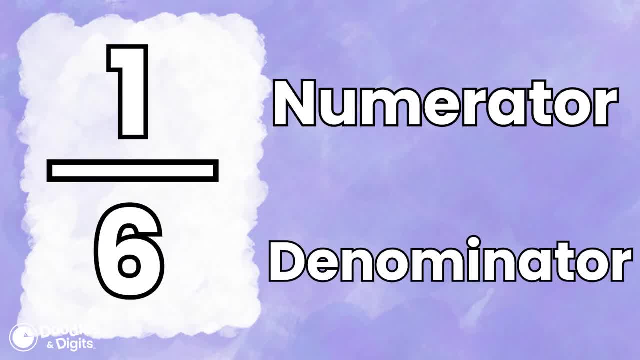 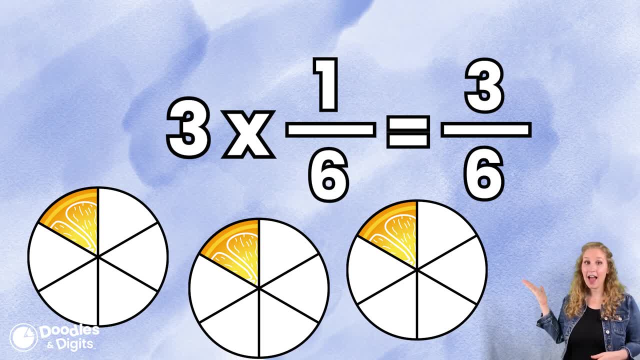 the numerator tells us how many pieces we have and the denominator actually tells us how big the piece is. we're not changing the size of the piece, we're just changing how many pieces we have. when you're multiplying fractions by a whole number, it's similar to multiplying whole numbers. 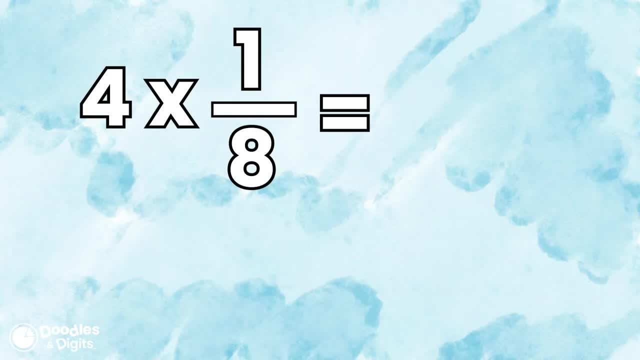 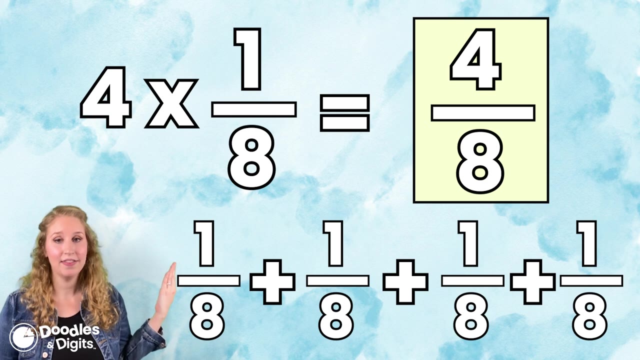 you could think about it as repeated addition. all right, let's see if we can solve this one with repeated addition four times one eighth. so we're gonna add one eighth four times one eighth plus one. eighth plus one eighth plus one eighth equals four eighths. the denominator doesn't change. 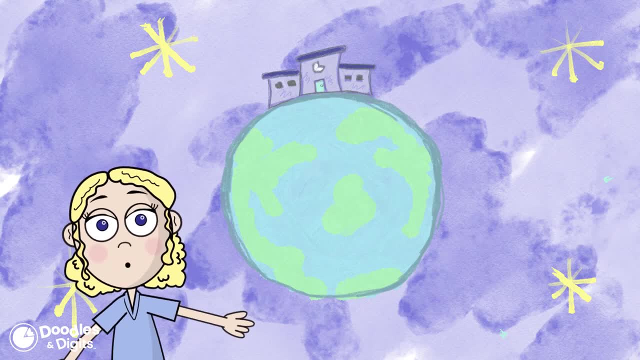 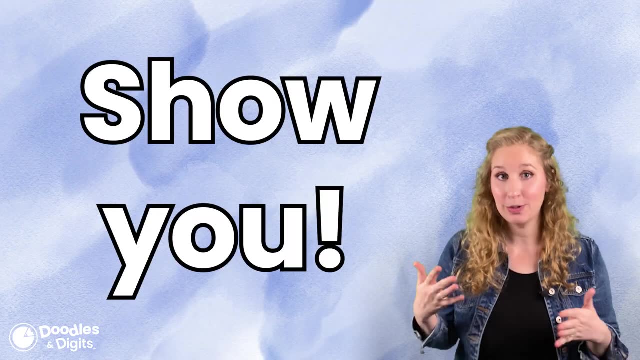 gets of the pizza. As you can see, there are multiple ways that you're going to use this in real life situations. All right, so I'm going to actually show you how to multiply a fraction by a whole number, and I want you to see what's going on. Let's look at this problem right here. 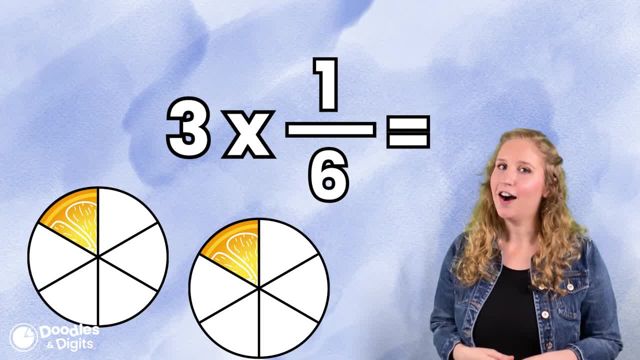 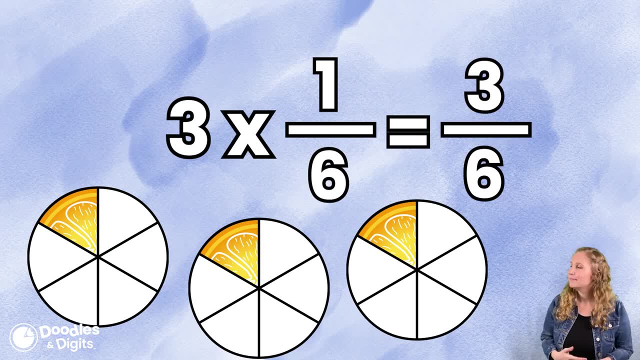 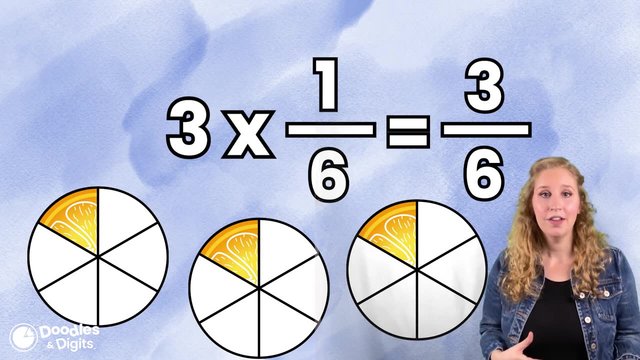 I'm going to solve it All right. what do you notice? What am I multiplying and what's staying the same? What's going on with the models? you might have noticed, when we multiply a fraction by a whole number, we're gonna actually multiply. 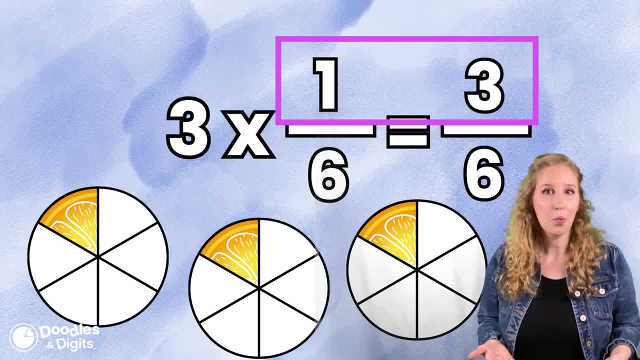 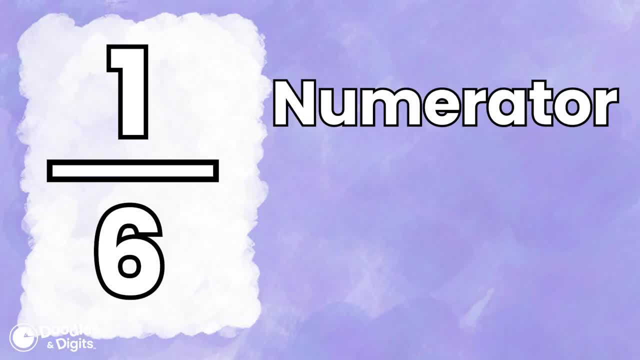 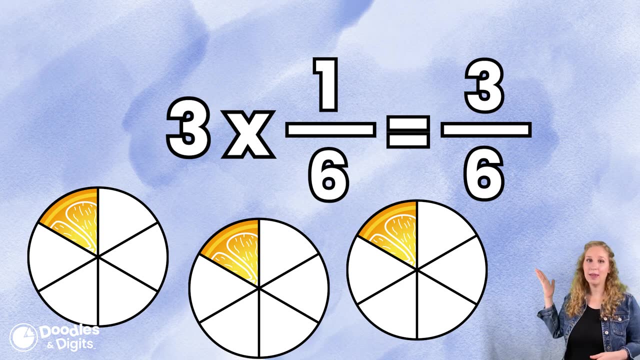 the numerator and keep the denominator the same. why? well, because when we look at fractions, remember, the numerator tells us how many pieces we have and the denominator actually tells us how big the piece is. we're not changing the size of the piece, we're just changing how many pieces we have. 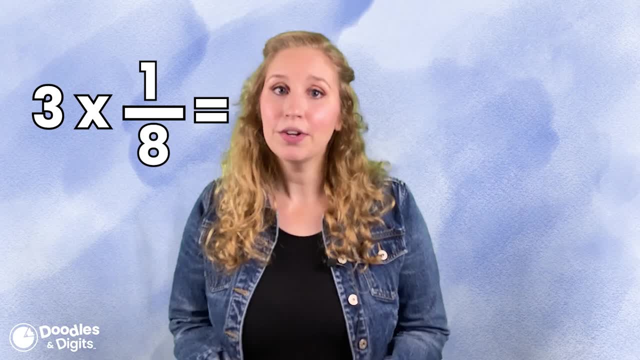 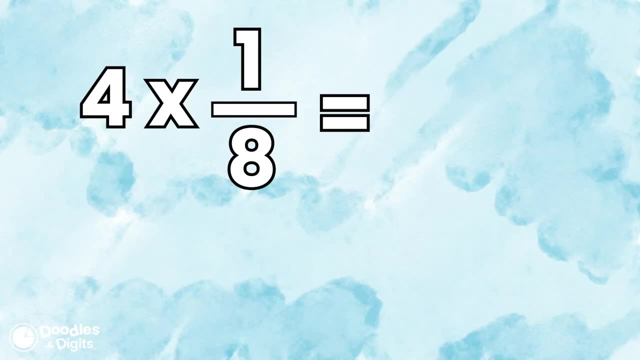 when you're multiplying fractions by a whole number. it's similar to multiplying whole numbers. you could think about it as repeated addition. all right, let's see if we can solve this one with repeated addition four times one eighth. so we're gonna add one eighth four times one eighth plus. 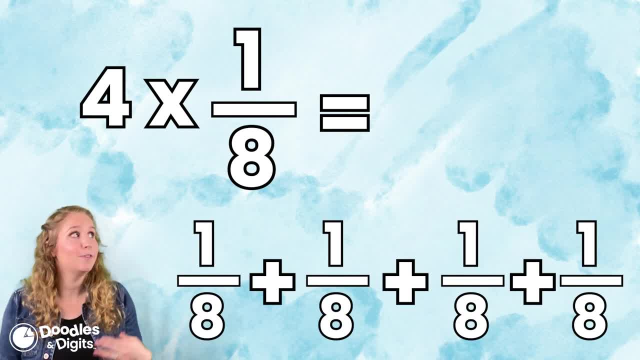 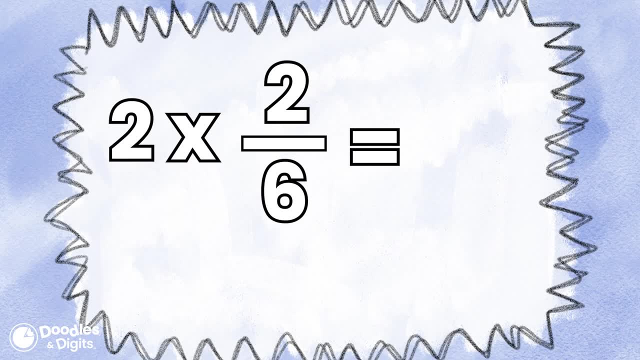 one eighth plus one eighth plus one eighth equals four eighths. the denominator doesn't change. all right, let's try a few more. two times two sixths- we're gonna first draw the model: two times two sixths is four sixths. four times one fourth. 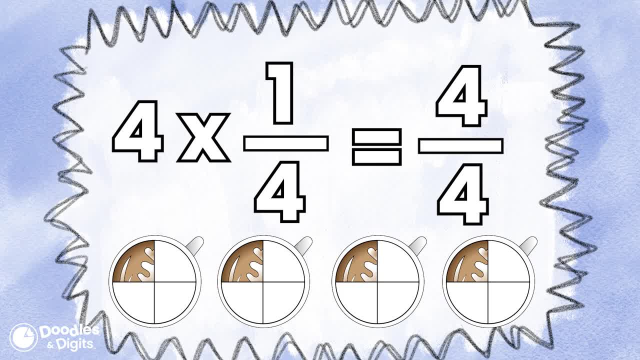 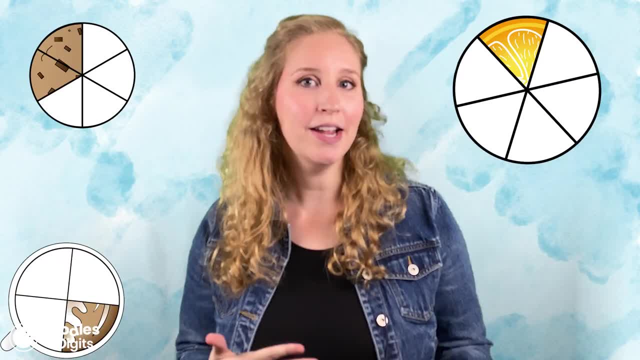 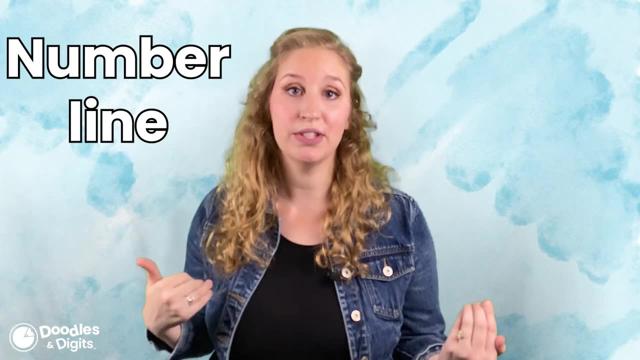 four times one fourth is four fourths or one whole. models are a great way to show your thinking and also to show your work, to go back and make sure that you didn't make any mistakes. all right, not only can you use models, you can also use a number line to multiply fractions. let's look at this number line right here. 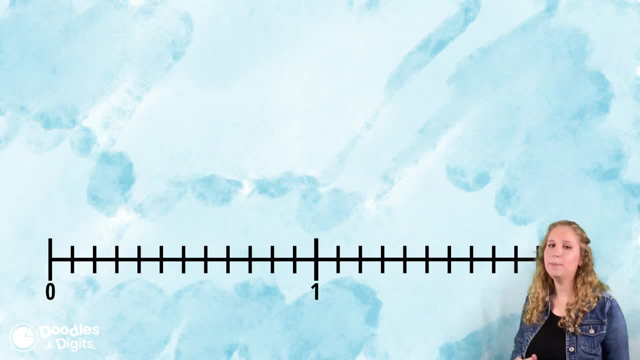 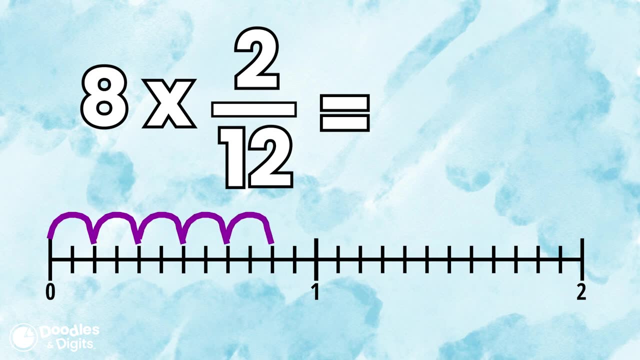 all right number line. let's see how can we multiply eight times two twelfths. all right, we're going to make eight jumps that are two twelfths each. where do we land? we land on sixteen twelfths or one and two twelfths.